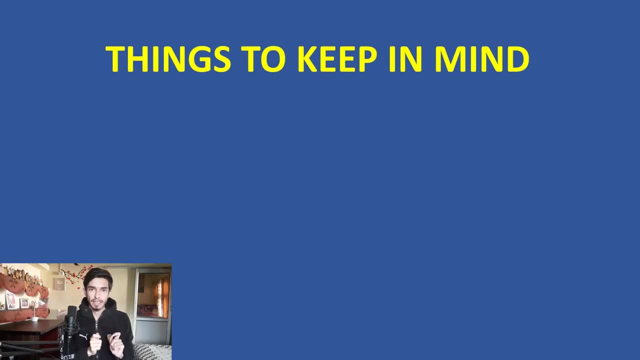 Now for solving a word problem. you need to keep these things in mind While reading the question. you need to see what are the unknowns in here and assign a symbol to every unknown you see. And the second thing you need to see is what is relating that unknowns. Using those relations, we will convert this. 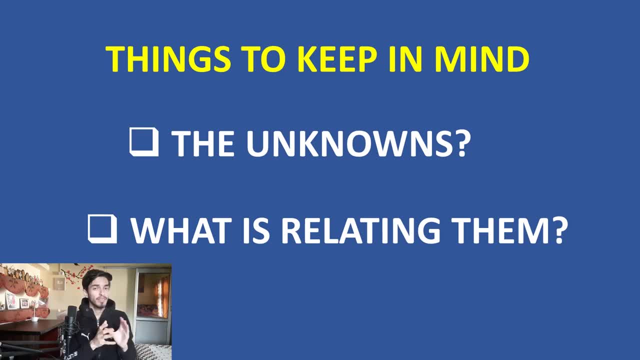 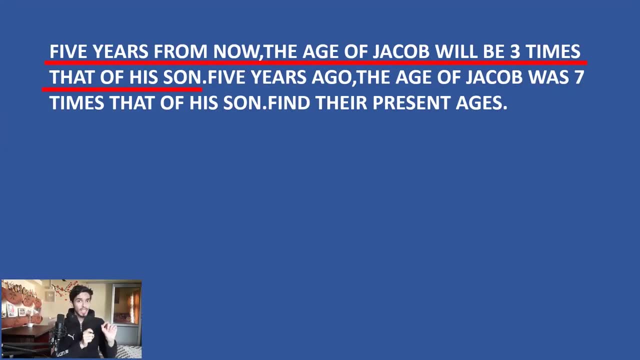 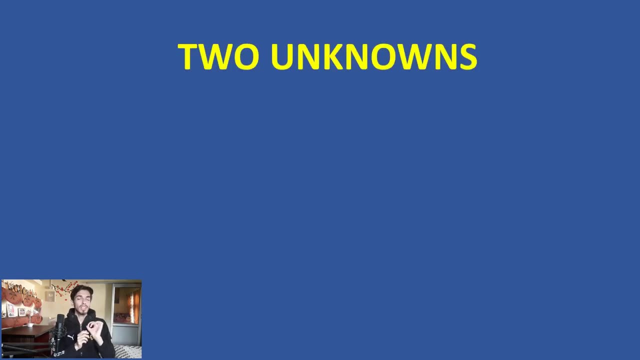 word problem into a mathematical equation, and then we will solve our question. Okay, so let us read this question carefully. 5 years from now, Jacob's age will be three times that of his son's age. now see, we have two unknowns here, which are Jacob's present age and his son's present age. so let us 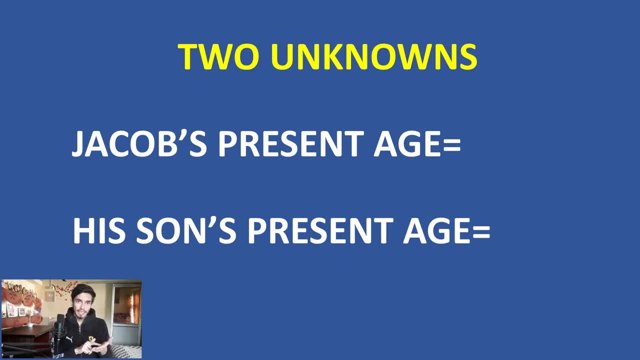 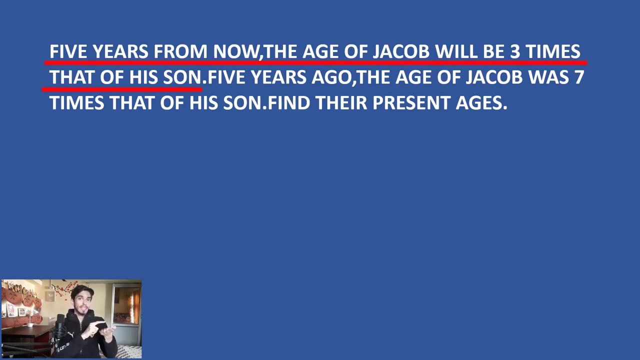 assign symbols to them. Jacob's present age is X and his son's present age is Y. okay, this was step 1. now what is relating these unknowns in here? they are saying five years from now, the age of Jacob will be. so they are saying Jacob's present age X plus 5, three times that of his son's age, which is equal to. 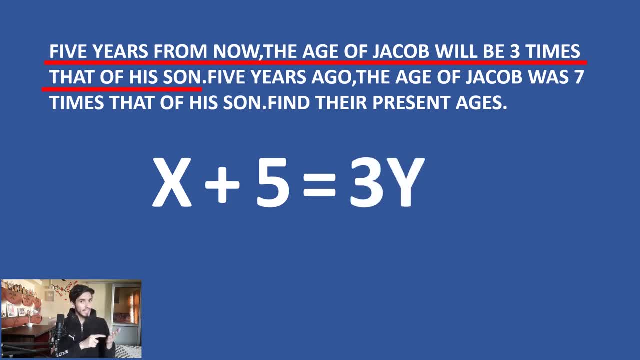 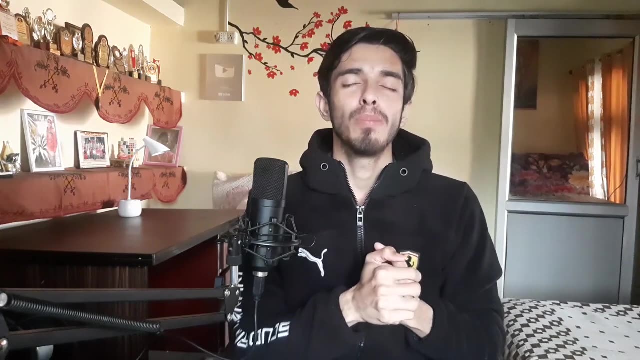 three times son's age is Y, right. so our equation is: X plus 5 is equal to 3y. this is correct right now. if you are saying yes, it is correct, then you have fallen into the trap of this word problem, because most of the word problem set traps to you that you can fall in. so in 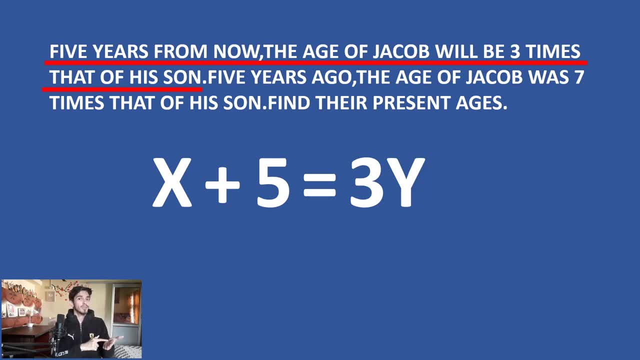 here. read this line again carefully: five years from now, Jacob's age will be three times that of his son's age. okay, so see, we have added five years in Jacob age, but on the other side we just multiplied three with his son's present age, but five. 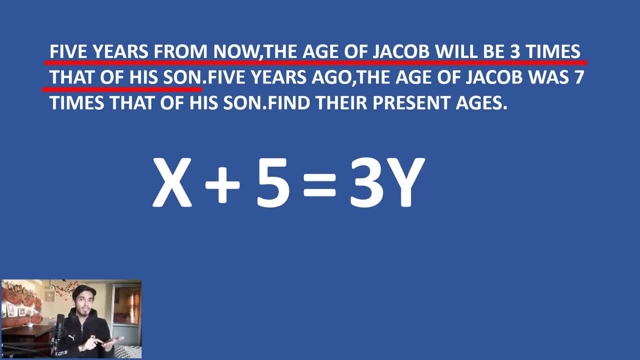 years from now, his son's age will also increase three times that of his son's age. but five years from now his son's age will also increase by five. so the statement is not saying: five years from now, Jacob's age will be three times that of his son's present age. they are not saying. they are saying: 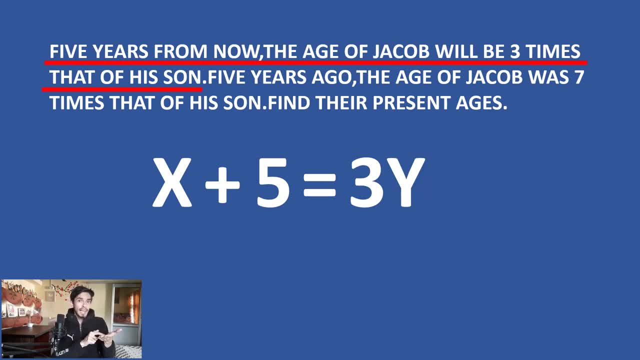 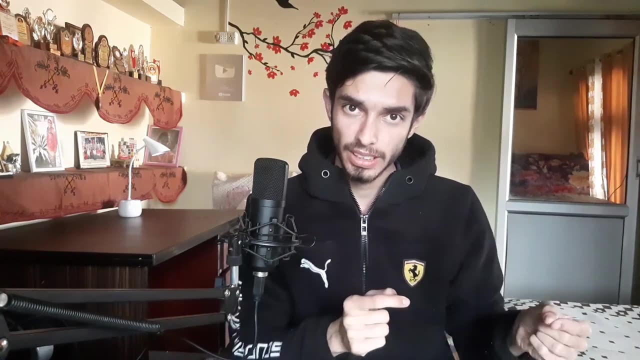 his son's age. so the real equation will be: X plus 5 is equal to 3 times Y plus 5, because we need to add those five years to his son's age too. so from this you can learn how important it is to read the question carefully and understand the. 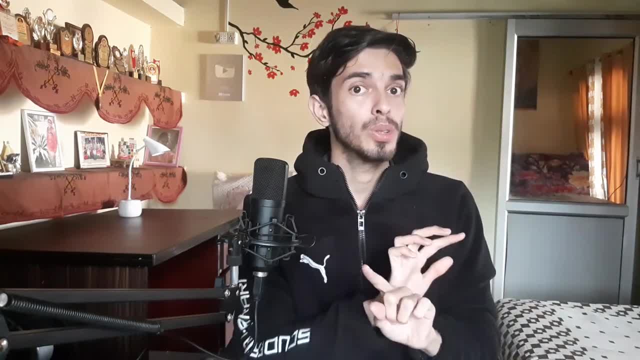 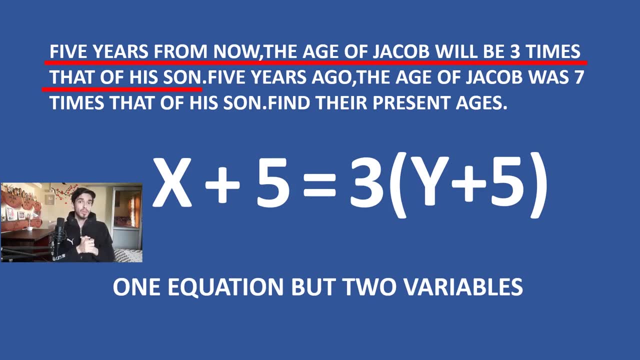 question and always remember there are traps in word problems you should never fall for. okay, so now we have one equation. but see, we have two variables. and always remember that to solve an equation with n variables we need an equation. so see, in here we have two variables, X and y. so we need at least two equations to find the 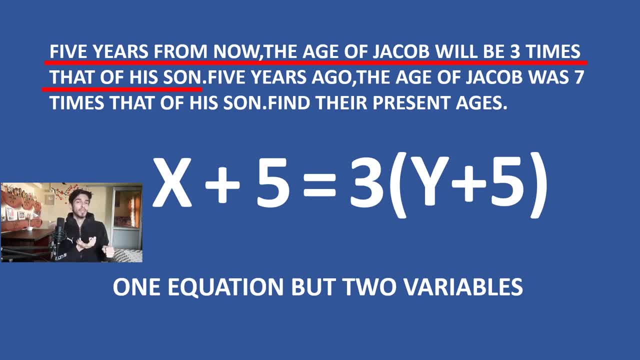 value of X and Y, which are our answers. so now let's read the question further. five years ago, Jacob's age was seven times than an adult age. relax, we just need to read the question further. five years ago, Jacob's age was seven times than an adult age. 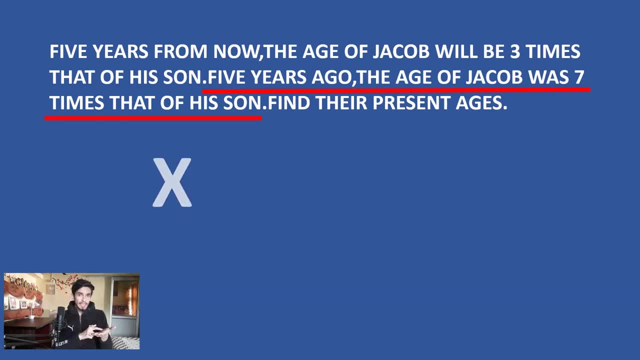 that of his son's age. so x minus 5 is equal to 7 times y minus 5. so never fell for the trap of 7y. it is y minus 5, because they are not saying the son's present age, they are saying the son's age. 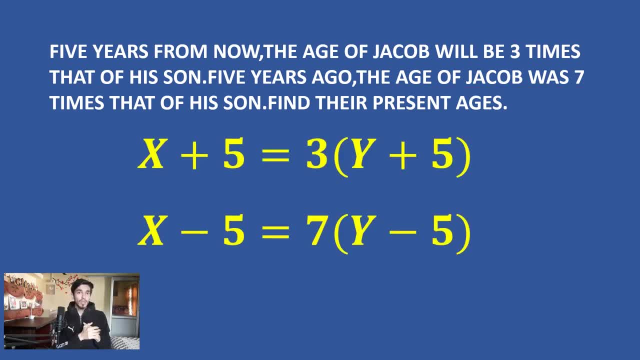 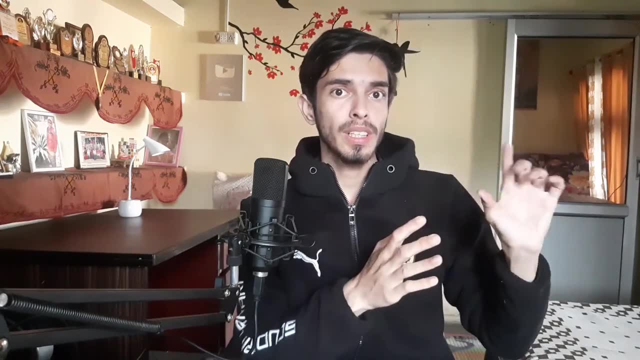 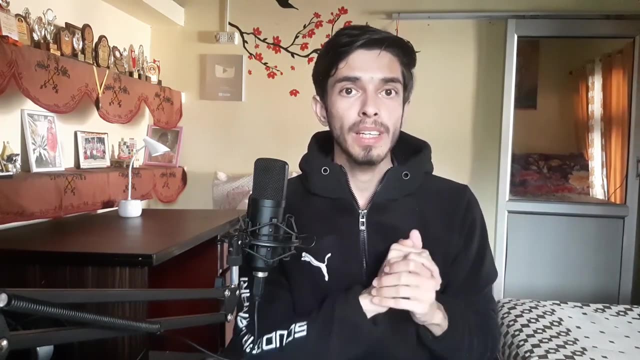 okay. so see, we have two equations in here, and all the information that can be extracted from the question is in these two equations. now one thing: i want to tell you that if you can convert a word problem into a math equation easily, you can solve any word problem. okay, now another thing. 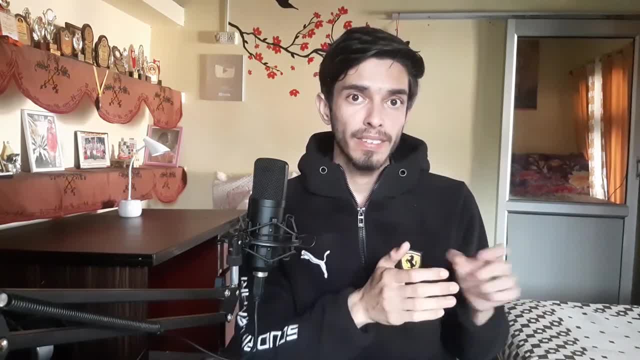 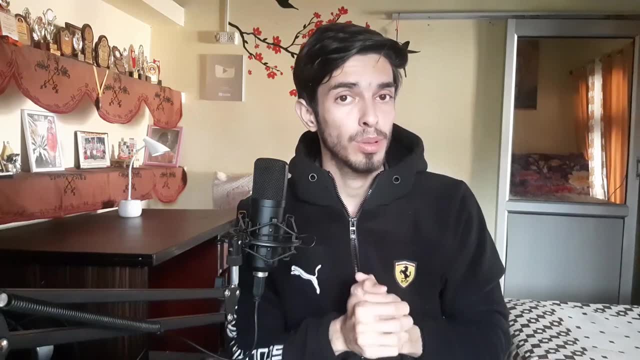 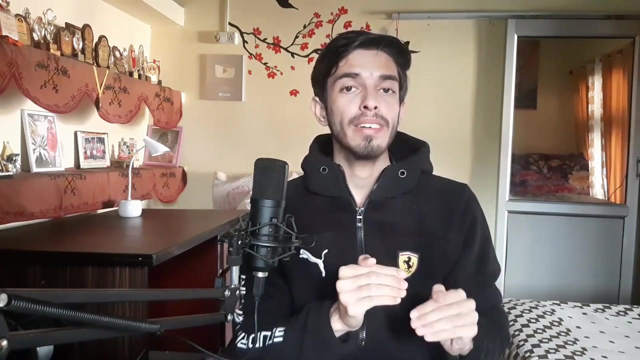 that i want to tell you is that sometimes this happens, that we have less equations but more unknowns. then look for more information in the question, because every word, problem, question in one way or another provide enough information to get to the answer. so if you don't have enough, 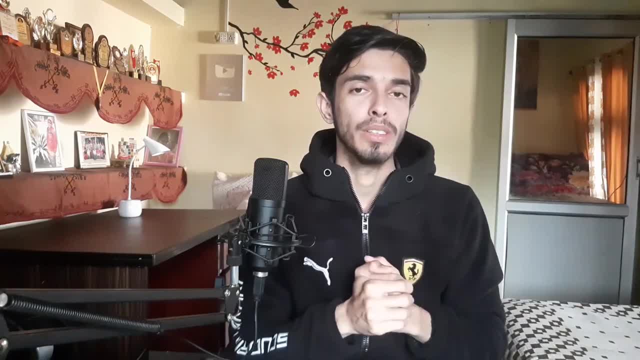 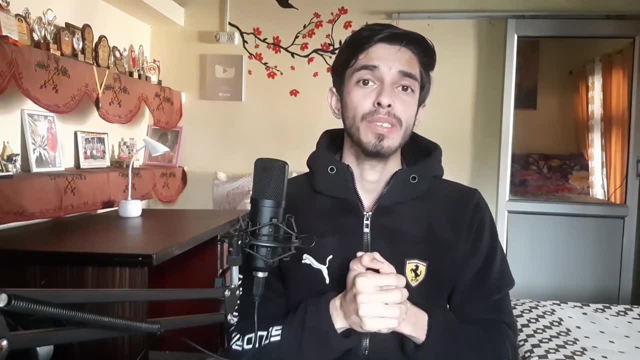 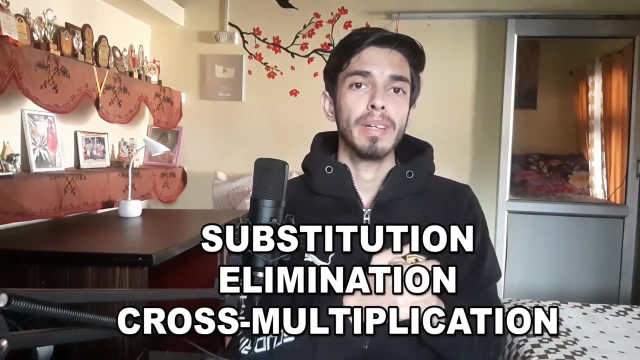 equations or more unknowns, then look for more information in the question. for now we have enough equations to get to the answer now. there are many ways to solve linear equation. in math there is substitution, elimination, cross multiplication, and we can also use these three methods mixed. so in this equation we can clearly see if we subtract these two, we can. 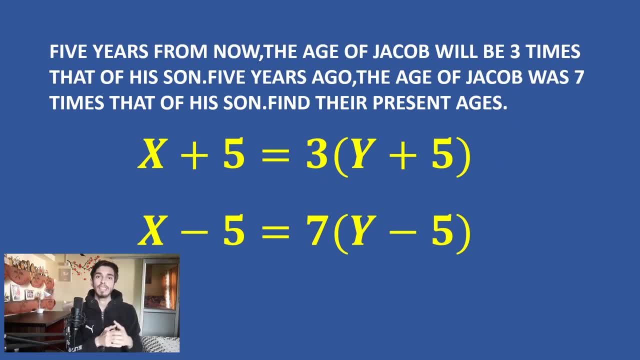 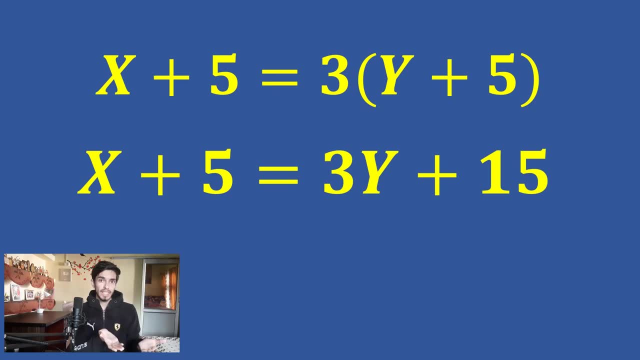 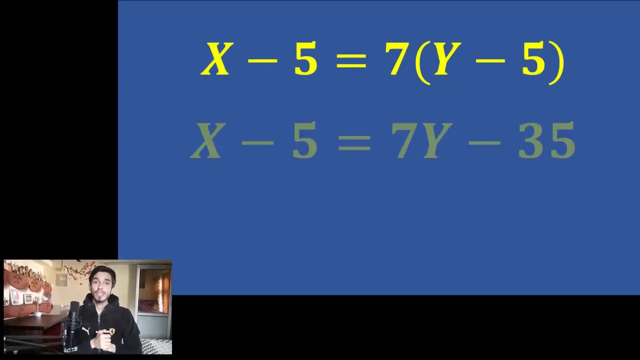 clearly eliminate x, so i will use elimination method in here. so now let us simplify this equation a little bit. which are x plus 5 is equal to 3y plus 15. now take this to this side, so we get x minus 3y minus 10 is equal to 0, and similarly for the second equation, we get x.